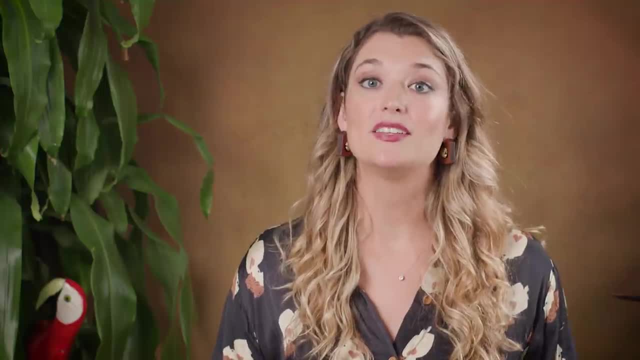 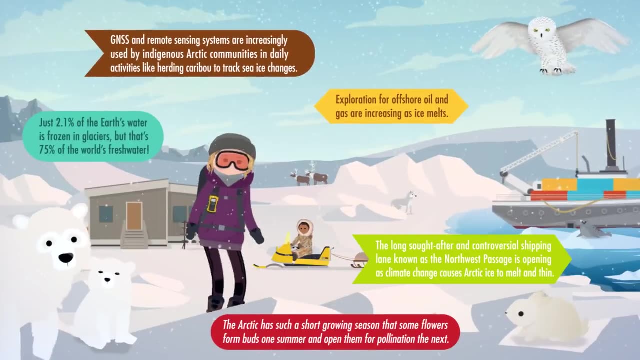 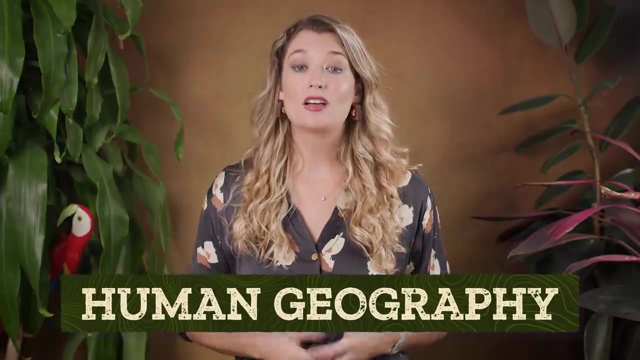 how people, power and economics combine in the world, impacting the human and non-human alike. I'm Alizé Carrère, and this is Crash Course: Geography. Human geography uses a combination of spatial, physical and social science to tell a complex 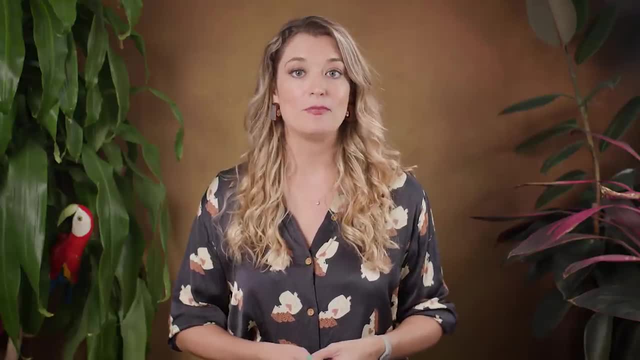 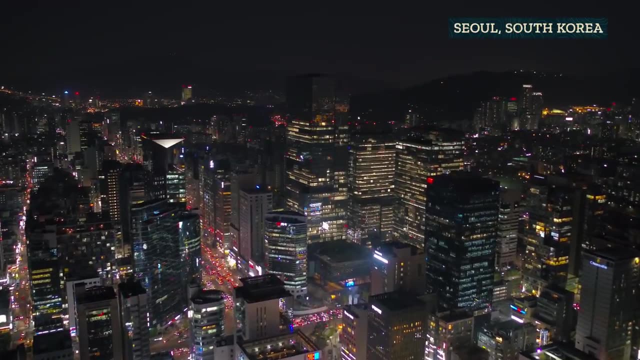 story of the world. This story focuses on the spatial patterns of people and how we've made sense of the places we inhabit, explore or create Like by giving them names And, as human geographers, we try to answer questions that pay special attention to the 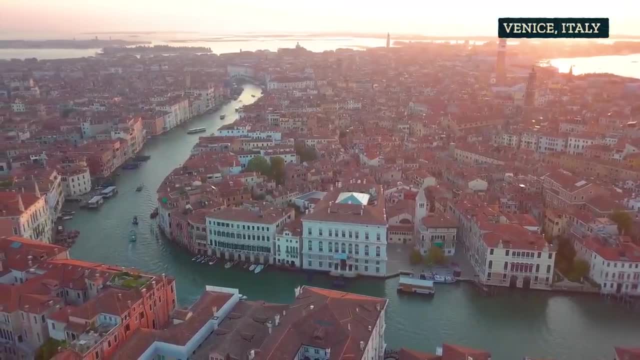 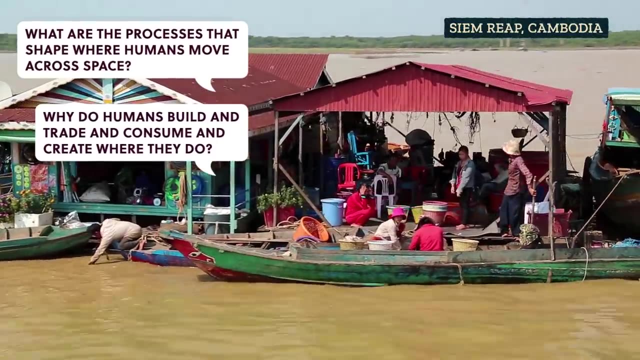 way people, power, money, buildings and so much more are distributed in the world? Like: what are the processes that shape where humans move across space? Why do humans build and trade and consume and create where they do, And why do those traits change across space? 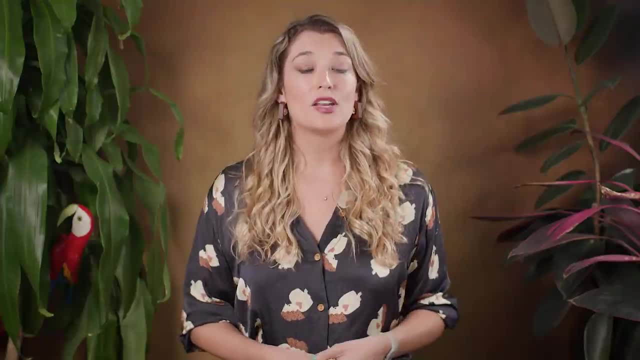 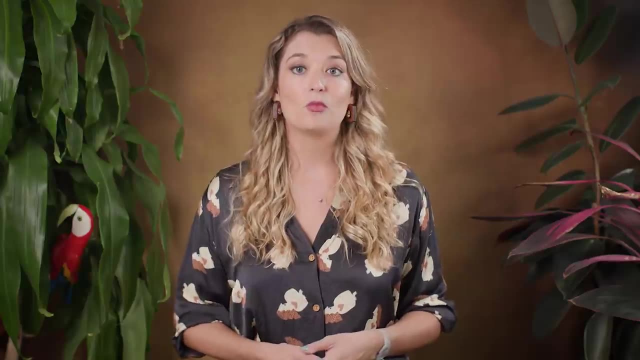 Why aren't all people and places just the same? We've actually already used human geography tools when we've considered things like the economics of banana plantations or the relationships between people or groups of people. one person or group has influence over another. This political power shows up when we talk about. 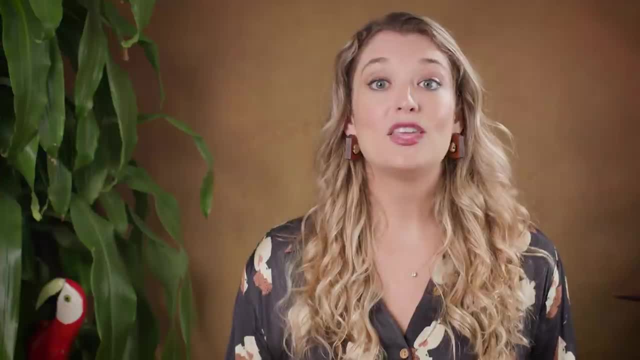 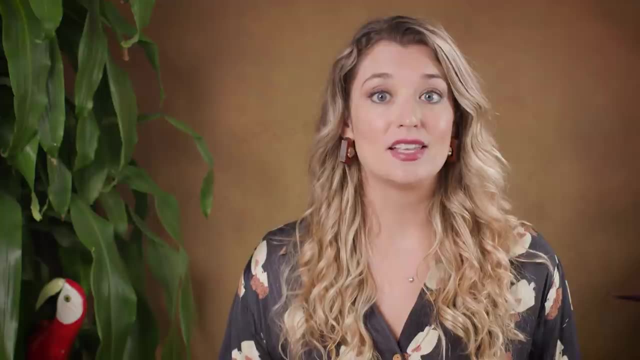 water access or the motivations for building in floodplains, for example. But the Earth is a big place and we could use a few more tools to fully tackle human geography, In addition to tools like maps and remote sensing or soil and vegetation surveys that give us data. 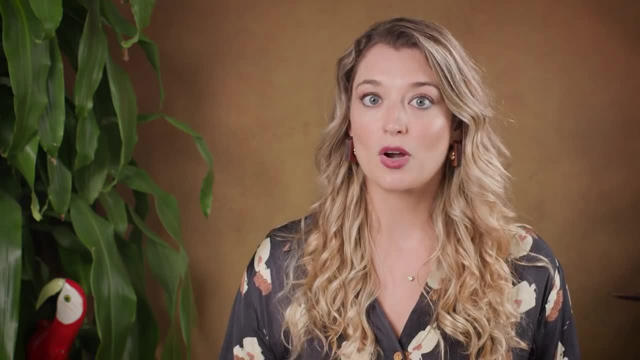 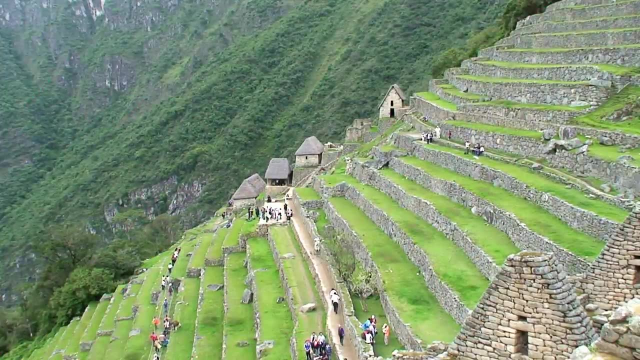 on what makes up our physical landscapes. the tools we'll need moving forward are actually concepts that help guide our thinking, Like the idea of place or the meaning we give a location and the sense of belonging we derive from constructing a place physically and in our minds. 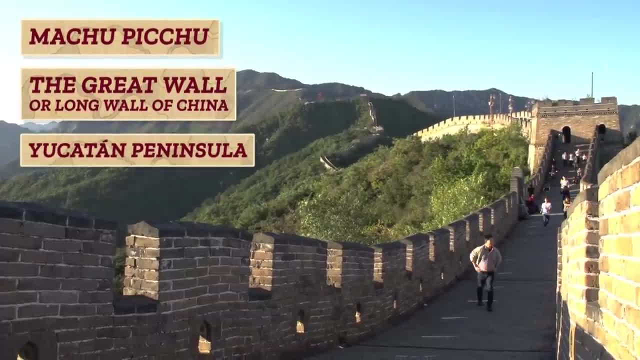 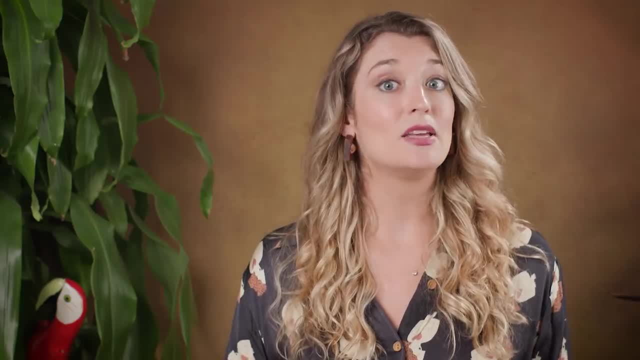 Machu Picchu or the Great Wall or Long Wall of China or the Yucatan Peninsula, or whatever name we give. a place is called a toponym and it's an important part of how we think about the place, Sort of like how my name is an important part of me. 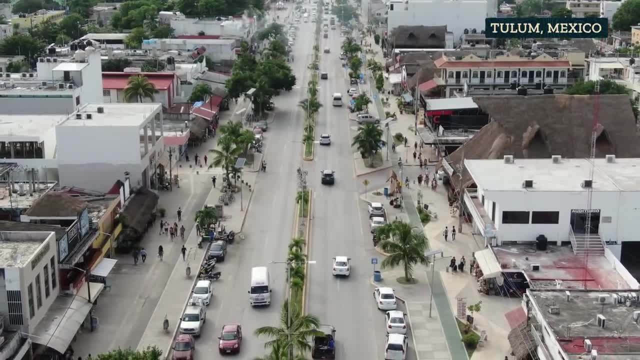 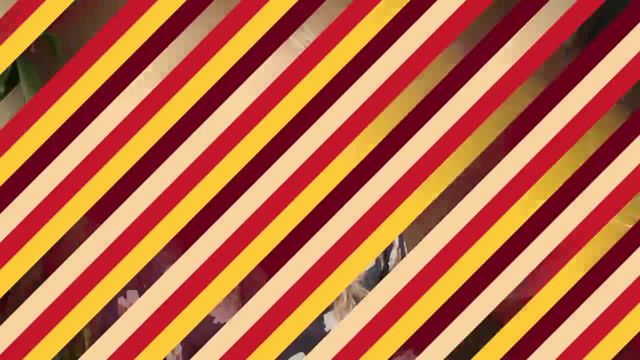 And if we dig into the history of a toponym, we'll learn the history of the location itself and see how it's changed over time and how different political and cultural forces work to create the place's identity, Like how I got my name and how it's changed. 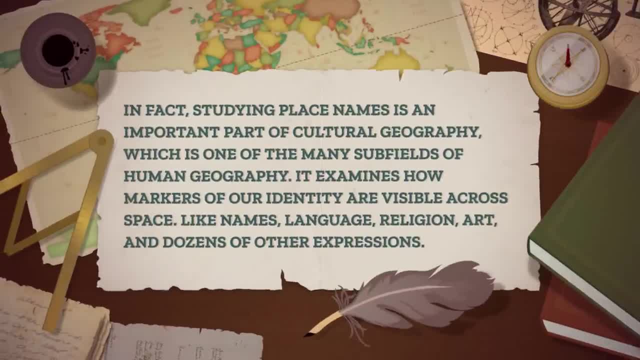 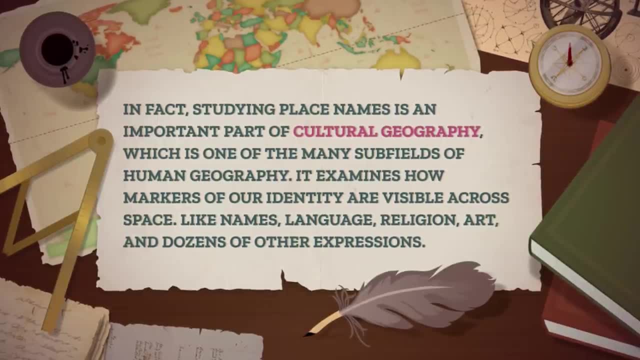 or what nicknames I've been given. In fact, studying place names is an important part of cultural geography, which is one of the many subfields of human geography. It examines how markers of our identity are visible across space, like names, language, religion, art and dozens of other expressions. 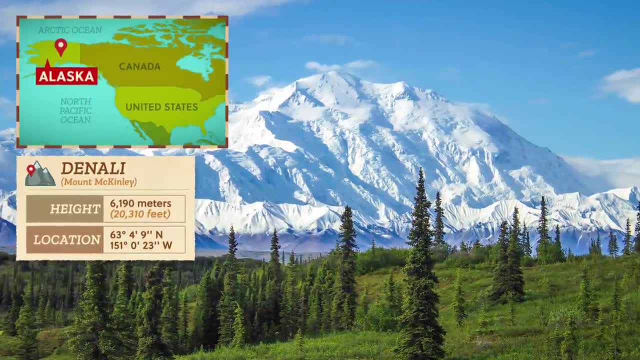 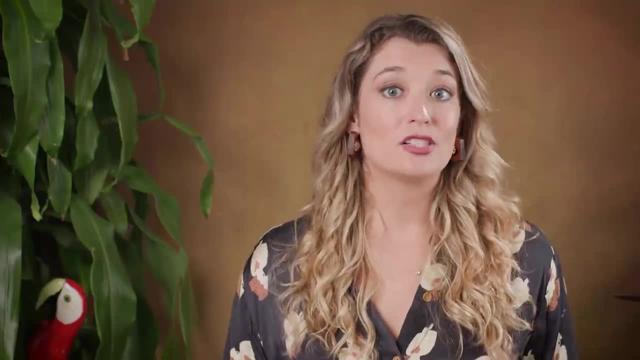 Like. let's look at the highest point in North America. It's a mountain reaching just over 6,190 meters high, known by some as Mount McKinley in what we now call Alaska. Even if we didn't know much else about this place or the space it's in the toponym Mount McKinley. 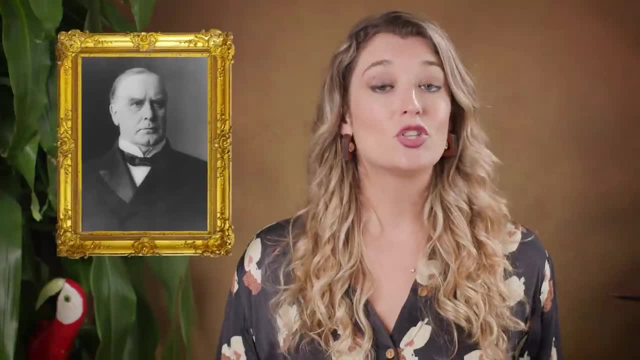 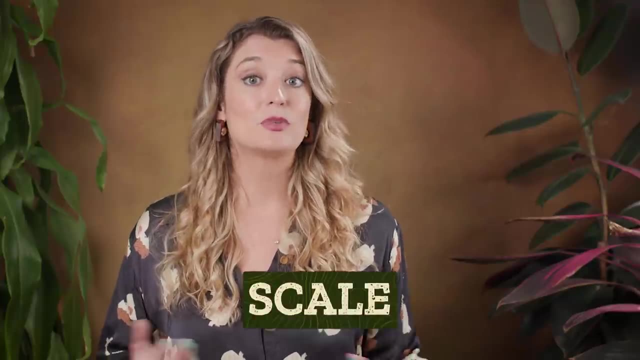 already gives us some historical and cultural context. It's a reference to the 25th President of the United States, which signals this is also a place in the US. Or we could draw on another conceptual tool, the concept of scale or the relationship a place has to the rest of the world. 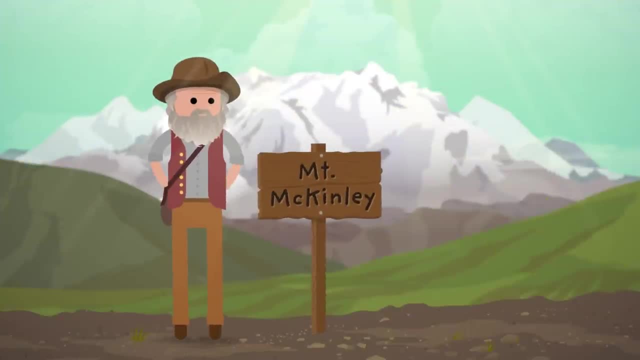 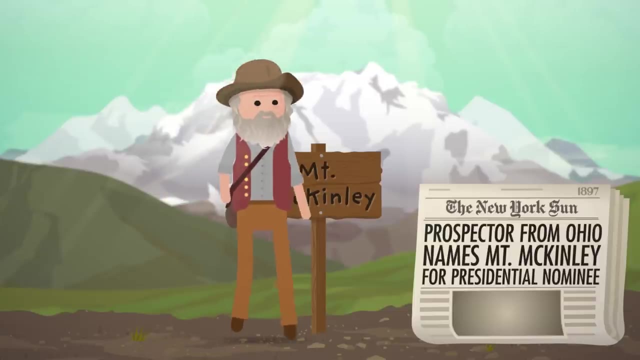 This mountain got the name Mount McKinley from a gold prospector from Ohio who wrote about it in the New York Sun newspaper in 1897, just before McKinley won the presidency. Other places in Alaska were also given names based on political figures from Ohio, other US states and the UK. 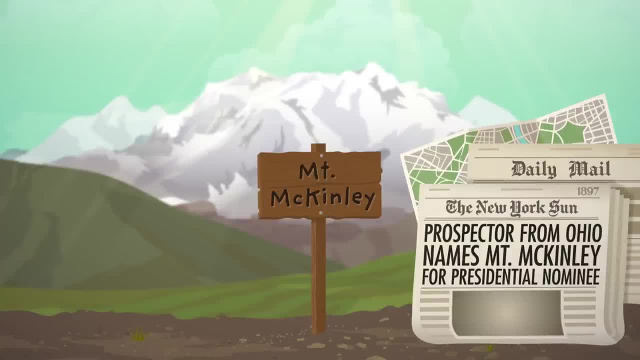 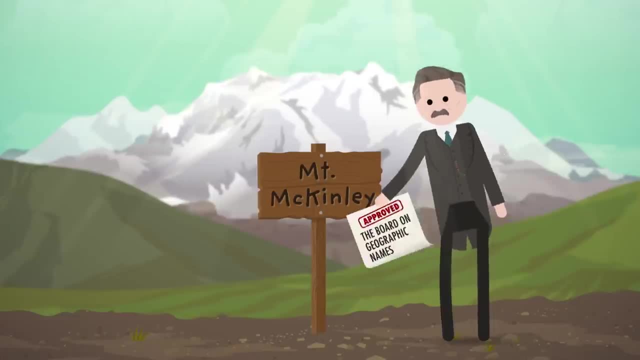 which were published widely in articles and used in official maps made by people not from Alaska. A few years later, in 1901, the Board on Geographic Names, which is a division of the United States Geological Survey, officially named the mountain Mount McKinley, And this was one of many name. 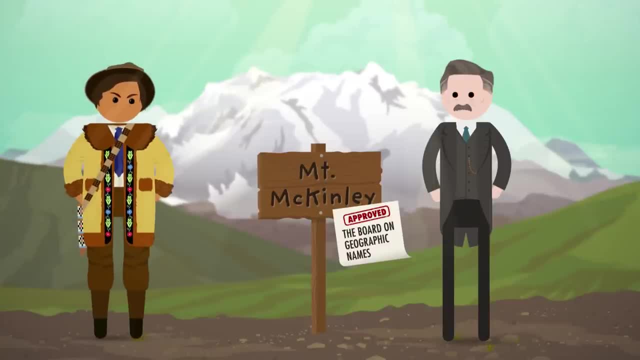 changes across Alaska, the US and around the world that moved the power to name the place from residents at the local scale to people with power at national and global scales, without representing local residents. That being said, as we'll see throughout the rest, 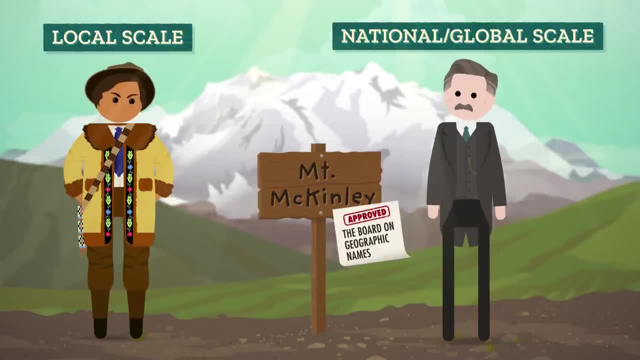 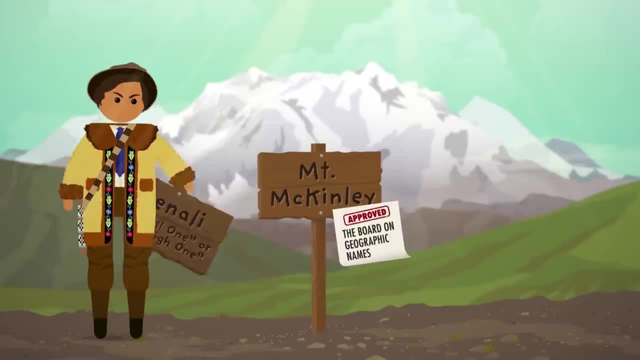 of this series. power has a way of changing hands a lot, and local residents aren't always united, But this majestic mountain already had a name. In fact, it had at least 30 names: The Athabascans who've lived in and around the upper. 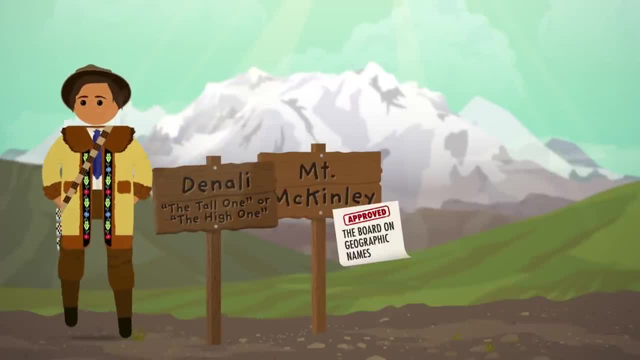 Kuskokwim River, often called it Denali, which reportedly means the tall one or the high one, And as early as 1906, there were writings that supported renaming this place Denali, But other indigenous nations who lived there had other names. 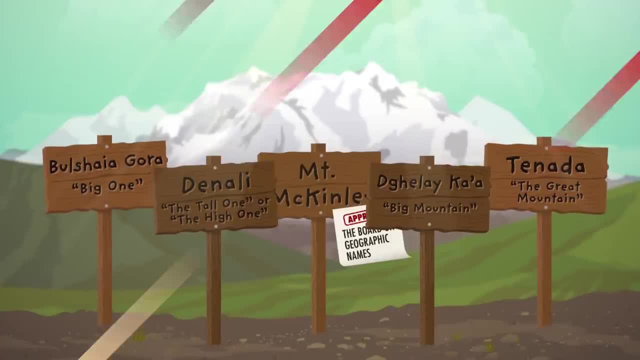 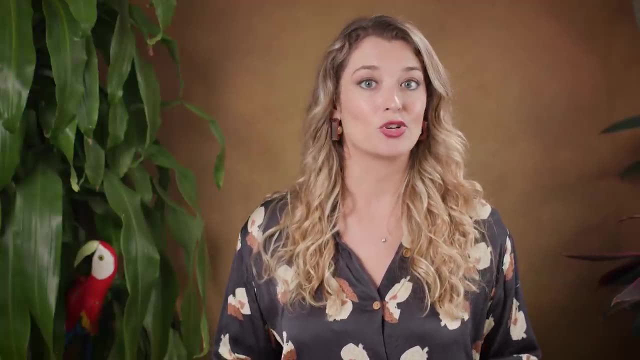 and so did people descended from what we now call Russia who also lived in this place. Names can also indicate power, as pop culture has explored many times, from urban legends to wizarding worlds, And in some cultures, like the Athabascans, you do not name places or things after people. 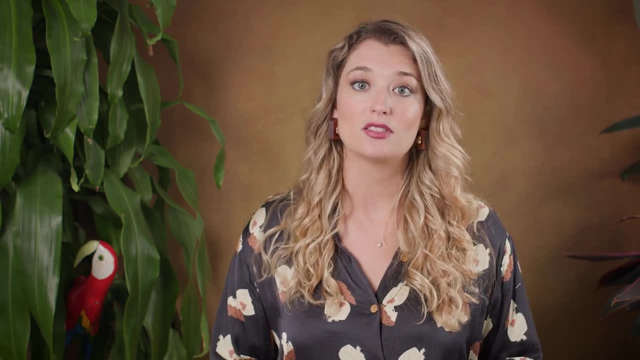 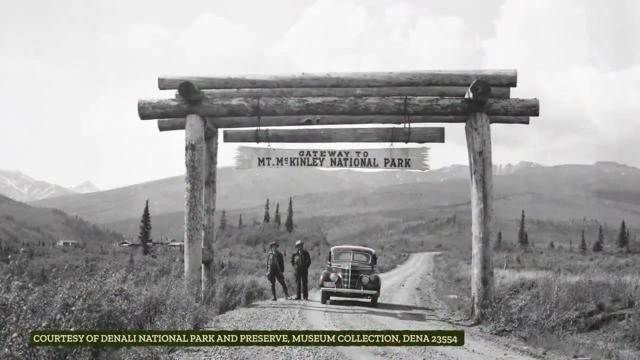 because place names are a way to describe the land and remember important details like resources or hunting techniques. Ultimately, the people advocating to put back the name Denali had less power and influence and could be ignored. In 1917,, the area around Denali became Mount McKinley National Park. 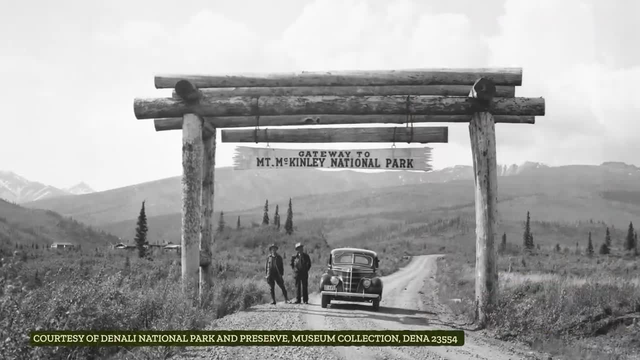 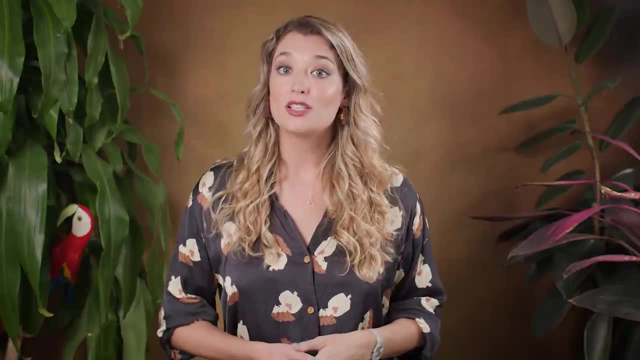 years before Alaska even became a US state, which redefined the place, and happened because of exactly the kind of uneven power dynamics human geographers study today All over the world. we can see the way that power is distributed across space, in part by the toponyms we give. 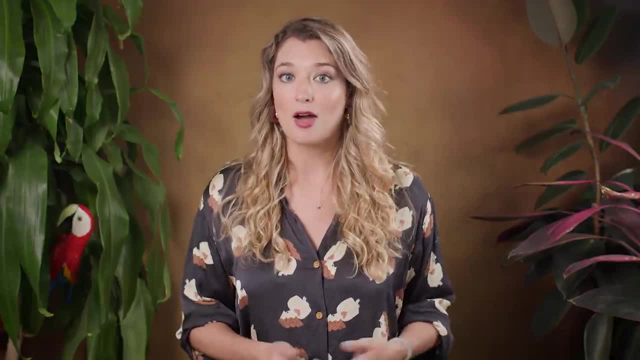 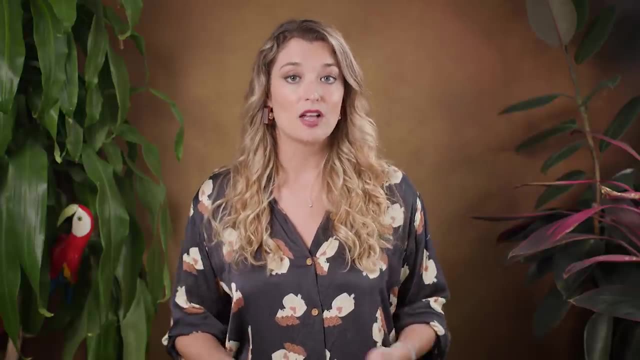 places, The names and landmarks that are revered tell us a lot about who has the power to name and create an image of a place. So what we call a place matters, because it sets up the way we imagine this space, like who owns it or what the culture should be, As Europeans settled throughout. 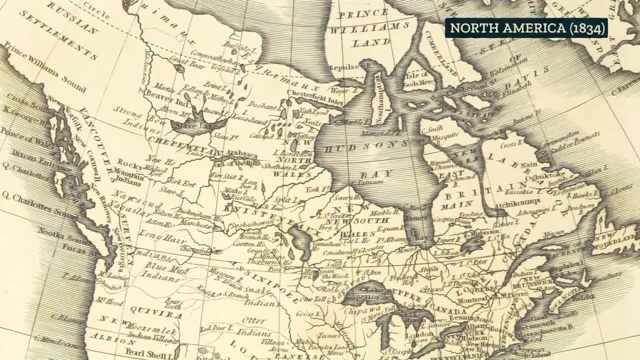 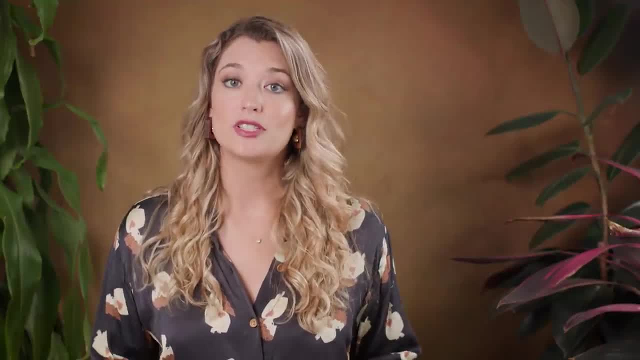 North America. they made strong efforts to claim the space as their own by renaming places and erasing the cultures and impacts of existing groups on the landscape. In fact, there's a third conceptual tool we can use to understand this place: The idea of a region, which is a way of grouping and classifying similar places. 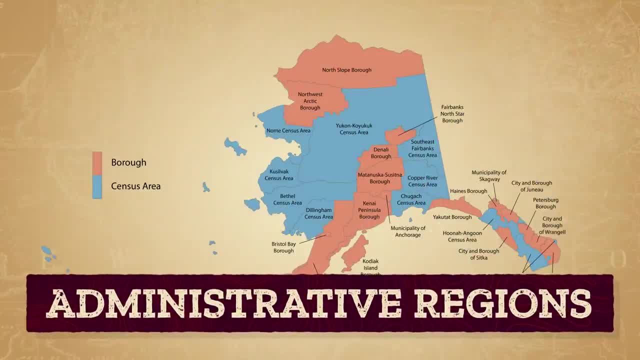 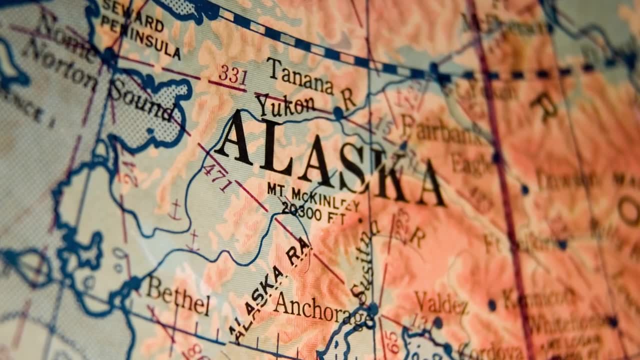 And there are different types of regions. Like many of the administrative regions or regions with legal boundaries within Alaska were imposed over existing boundaries of the nations who already lived there, And for Denali, or the renaming of many places known to indigenous peoples, the new name signifies a new perceptual region. 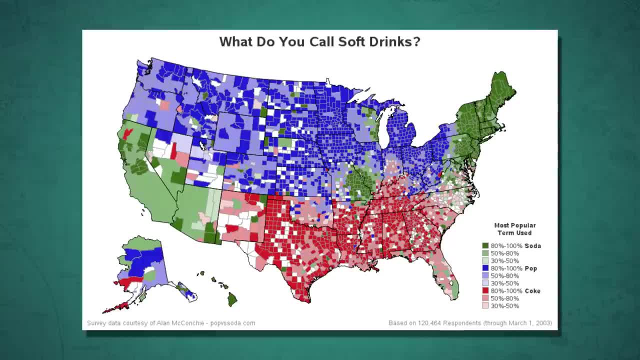 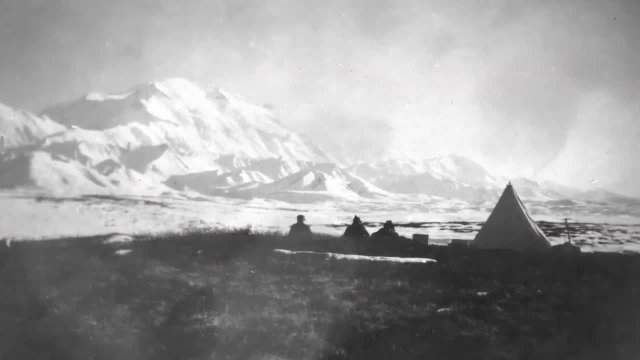 or a region that's united by how people think about or see it Like. a region that's unified around the language or cultural slang it uses or the team or cultural group. it's a part of The new name- created a relationship between Ohio and Alaska. It brought the mountain and Alaska. 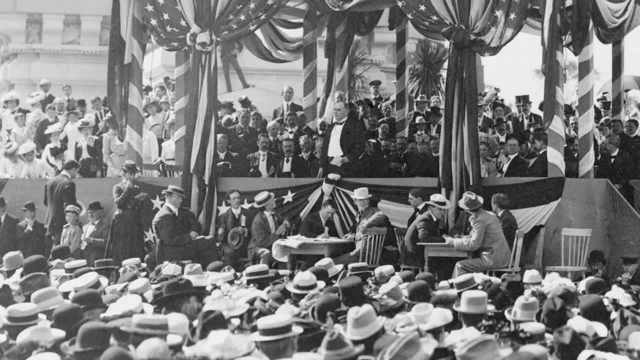 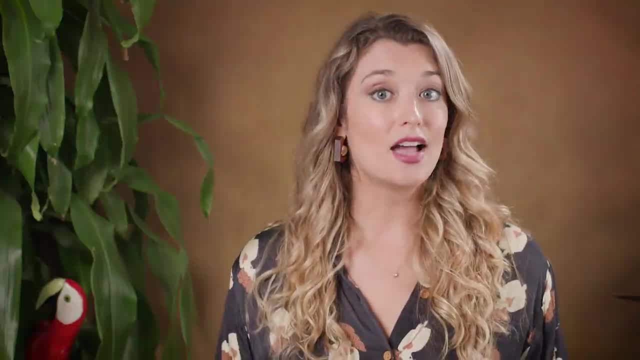 into the imagination of people in the continental US and possibly evoked a sense of patriotism by connecting Alaska to US politics, even though President McKinley had no connection to that place, Whereas at the time the name Denali created the perception this place has a culture. 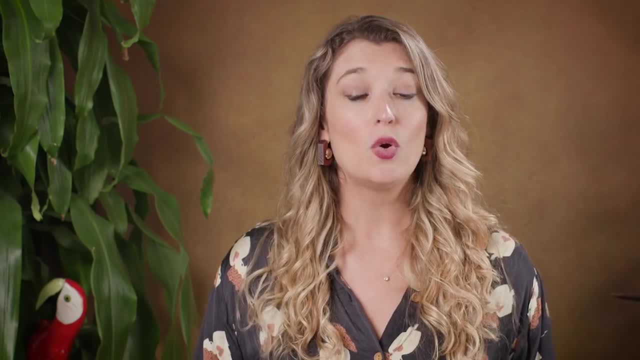 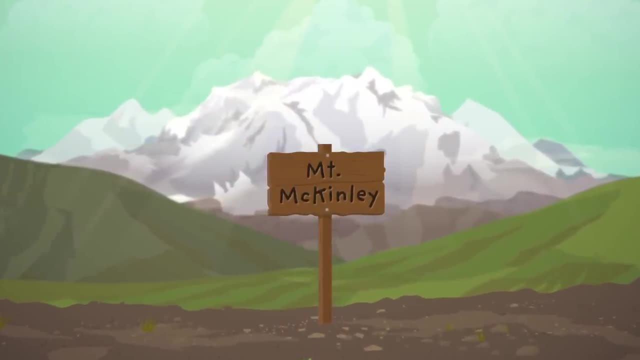 and history, foreign or other to most European Americans who held a lot of the political and cultural power. But the act of renaming also has power. That struggle that all humans feel to see their identity reflected back to them in their landscape is what motivated Alaska natives and 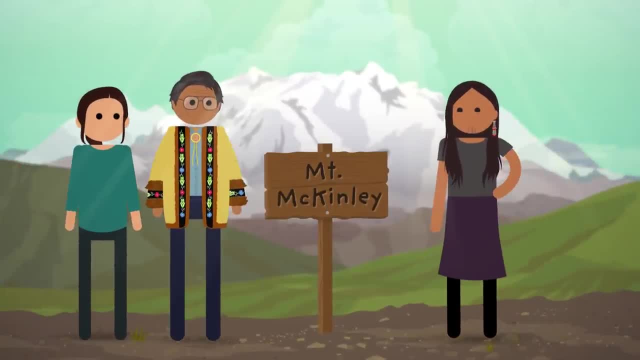 non-indigenous allies alike, to work for decades to change the name back In 2015,. that hard work paid off and this place was renamed Denali to reflect the peoples who have an ancestral connection to the land. We looked at the Denali name change and then re-change as cultural geographers. 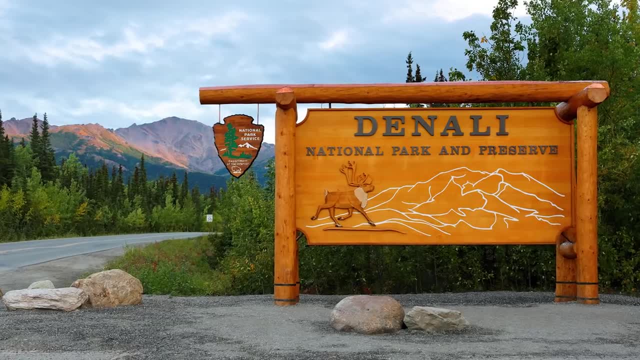 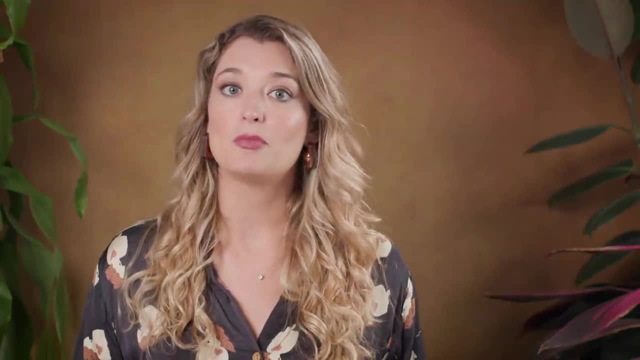 but there are other big parts of human geography we could also use to explore this place and space. Political geography studies the way that power shapes the landscape, like how here in Denali there was an uneven power between those in the Ohio and Washington DC and those in Alaska. And if we zoom all the way out to a global scale, 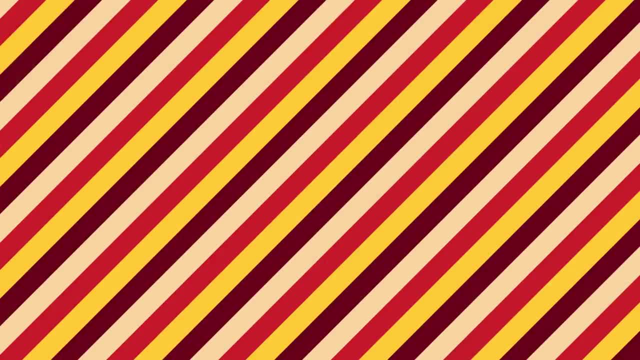 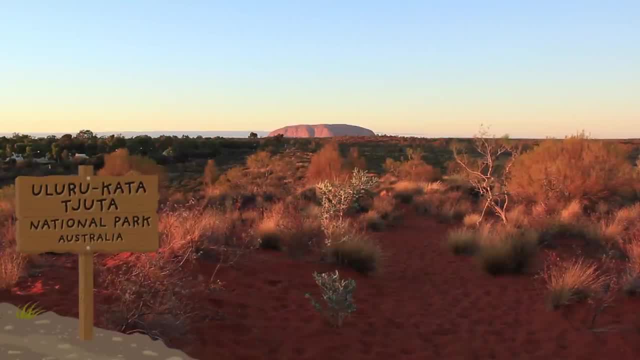 similar tensions over toponyms can be found in many other places, especially those that have been colonies or part of empires at some point in their history, Like in 1995, when Uluru-Kata-Chuta National Park in Australia was made official, ending the British name of Ayer's Rockmount. 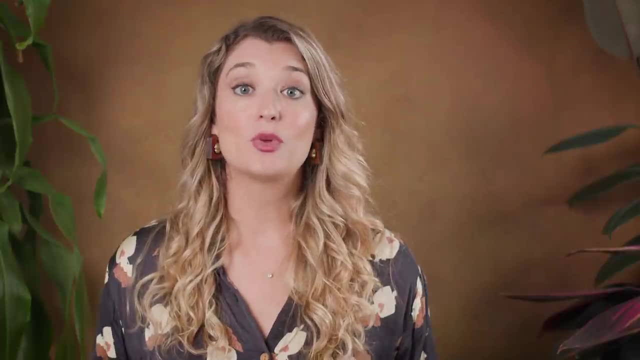 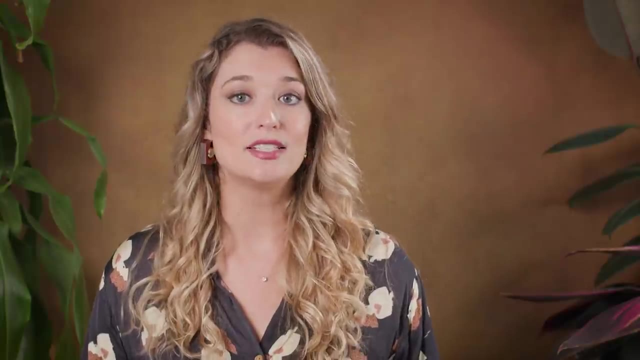 Olga National Park. Each place is complex, but as geographers we look for how places are connected. There are similar political and economic forces at work that help those in power show they have control over the identity of the place they're in. So restoring the names of places is an important 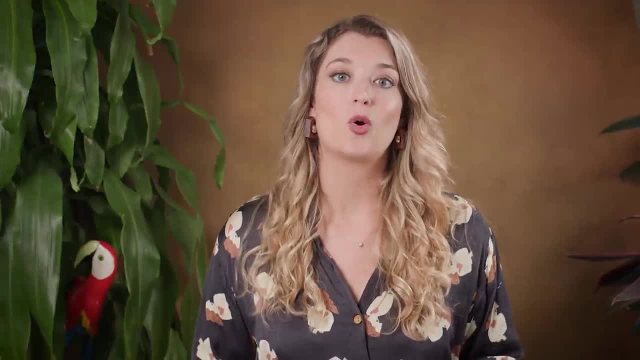 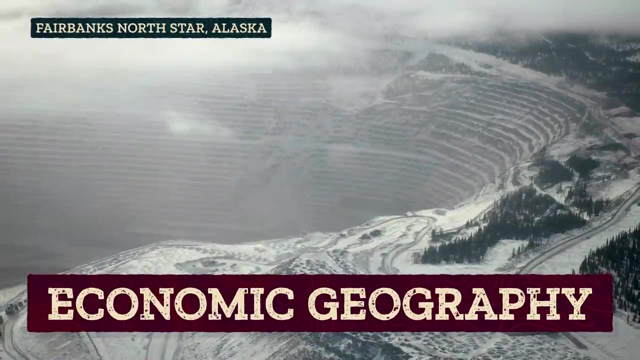 part of identity and cultural geography and important political work on the local scale as a way to push against regional and global powers. Or in economic geography, we study the uneven movement of economic opportunity, Like the way some opportunities like Alaskan gold mines. 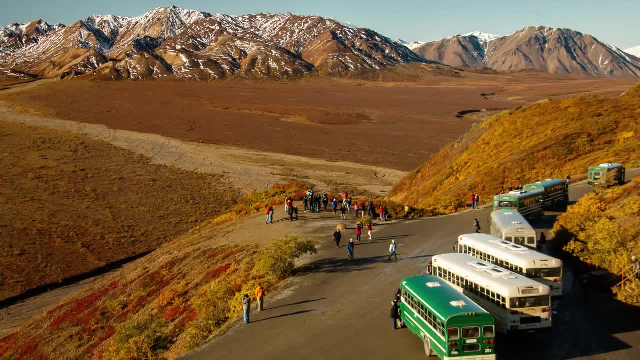 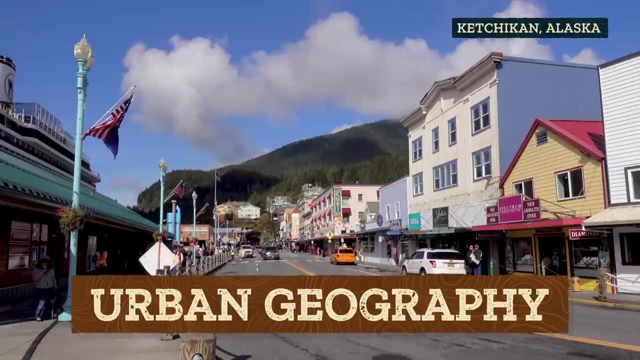 don't end up making the people living near those mines wealthy, Or the way the tourist economy may change throughout the national park depending on environmental, cultural or political factors. And finally, in urban geography we study the way humans build cities, Like what influences create the housing and industry. 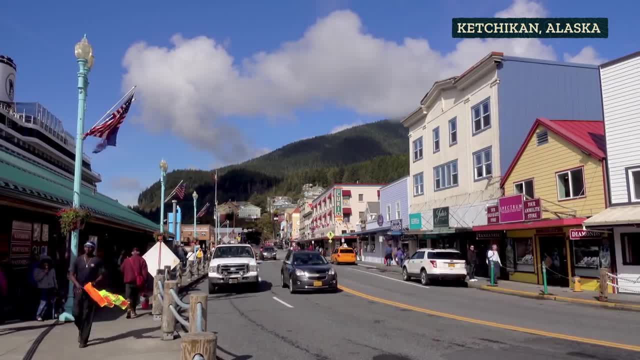 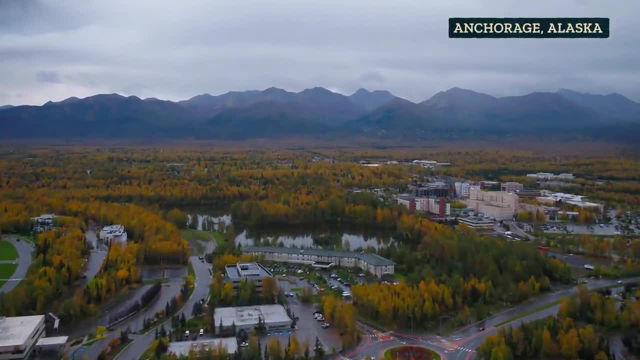 patterns or the ways we can plan spaces to maximize walkable communities and the relationships between urban and rural spaces, Which is still an important field in Alaska. As cities within the US grow, Alaska could have an important role as America's last frontier. Denali is just one example. 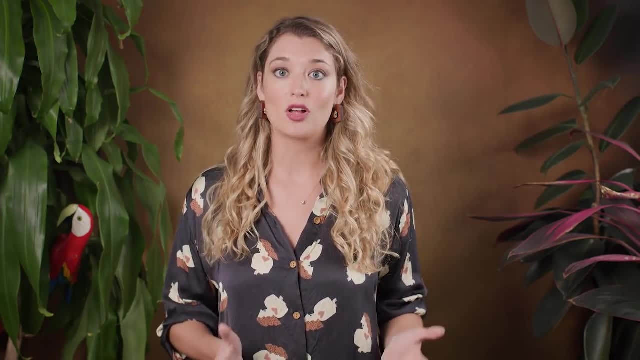 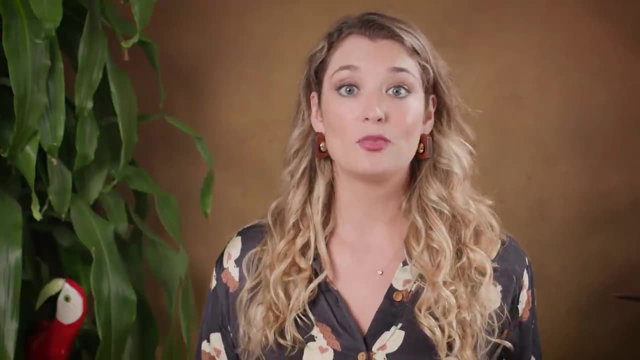 of a growing movement of indigenous and marginalized groups, asserting their cultural understanding of the places they have spiritual, cultural and legal rights to. There's power in place names. There's power in how we define regions, what's in versus out and who it includes. 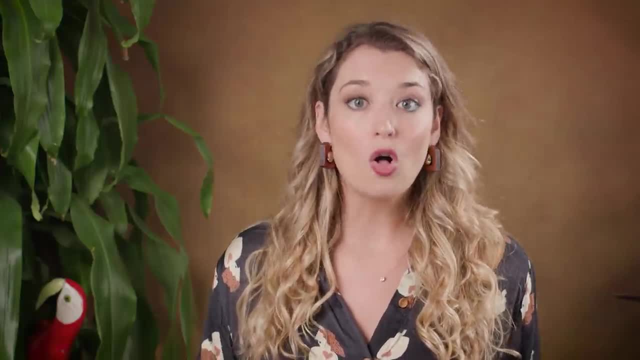 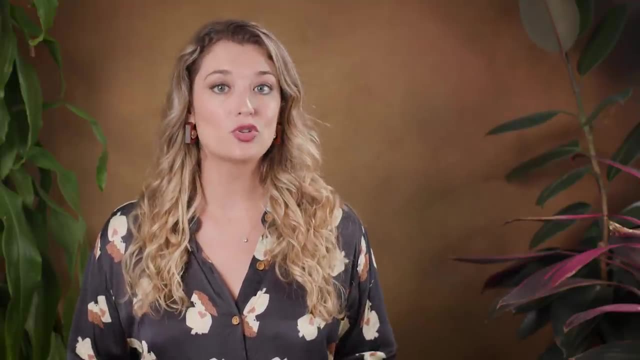 and who it excludes, Which is why we see struggles over place names all over the world. Our names shape our identities, And efforts to learn about the places we call home and their histories is part of the cultural and political work we can do to recognize who has been harmed by colonization and conquest.